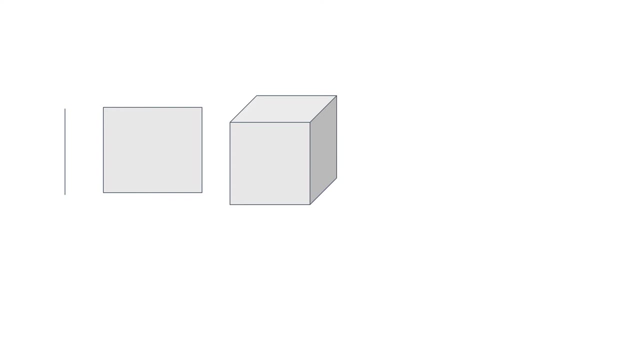 space increases exponentially. as the number of variables increases. In higher dimensional spaces it's harder to have a representative sample for every possible configuration of the parameters. This problem is also known as the curse of dimensionality. In reality, natural data have regularities and don't really use the entire parameter space. If 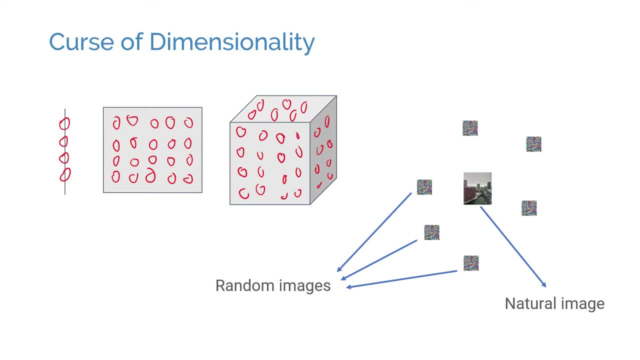 our data consists of images. for example, natural images make up only a small portion of every possible combination of pixel values. We can encode such inputs using fewer parameters by capturing a lower dimensional manifold that explains the data. In deep learning, dimensionality reduction is usually not done. 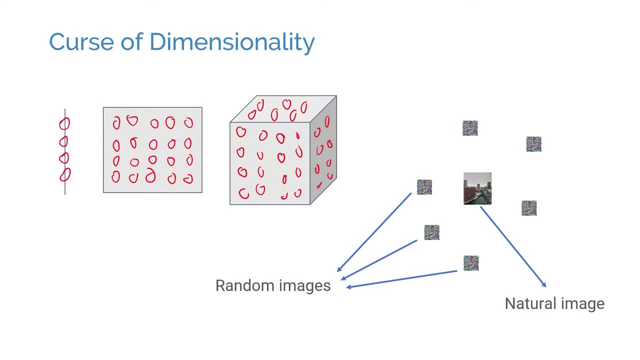 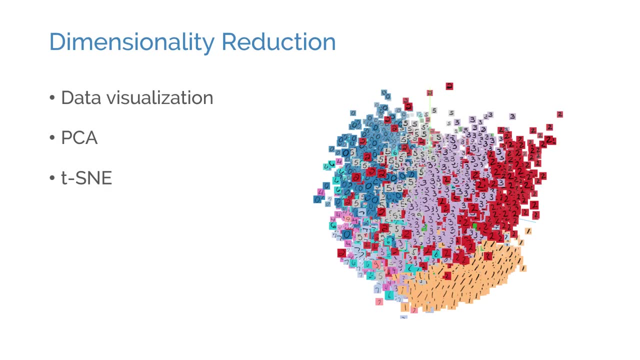 as a separate step, but the models learn compact representations within the model. It's still common to use dimensionality reduction techniques for visualization purposes, though For example, PCA or TSNE methods can be used to visualize data points with many dimensions in three-dimensional. 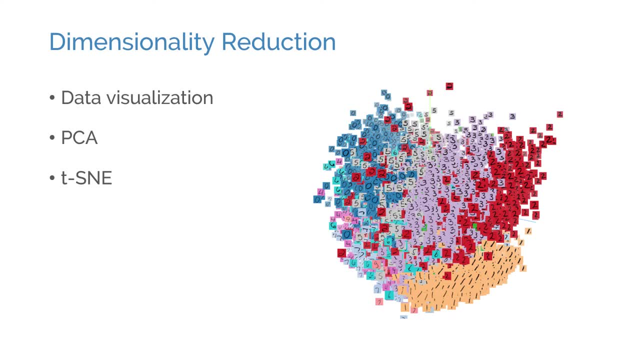 space Data visualization and traditional dimensionality reduction techniques are a little off-topic for this video, so I won't go into further detail, but you can find more information about them in the description below. Let's talk about how we can train a neural network in an unsupervised fashion. We need 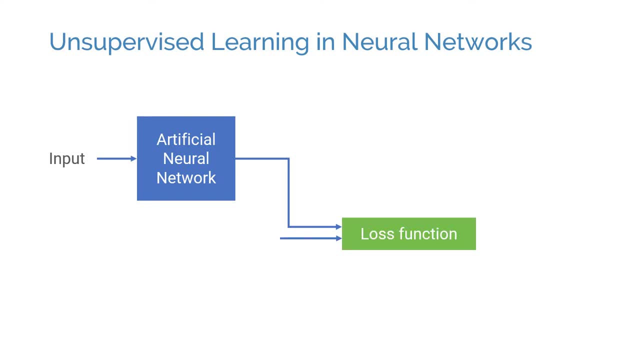 to define some sort of target to train a neural network. One thing we can do is to train a model to learn a mapping from the input data to the input data. Since the inputs and the outputs are the same, the model would try to reconstruct its input. These type of models. 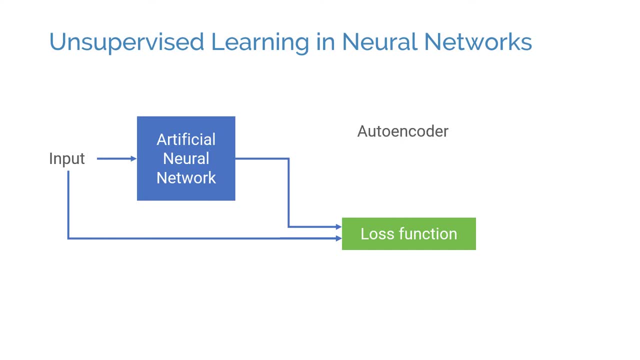 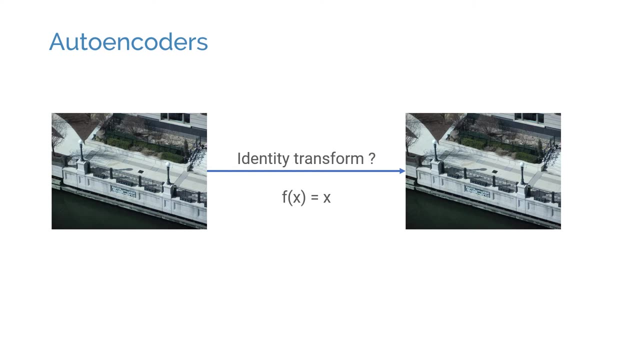 are called autoencoders. Of course it's trivial to define a mapping from the input to the input itself. Why do we even need a neural network to represent an identity transform? We don't actually want them to learn an identity transform. We want them to learn to represent. 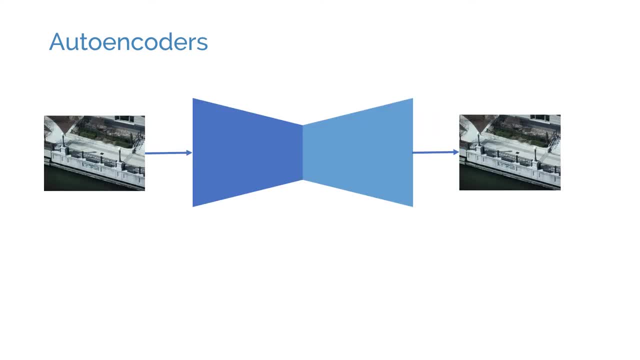 their input efficiently. A typical autoencoder is a feed-forward neural network that consists of encoder and decoder modules with a bottleneck in between. The encoder module distills the information into a lower-dimensional feature space. The decoder tries to reconstruct its input using the code, The inputs and the outputs. 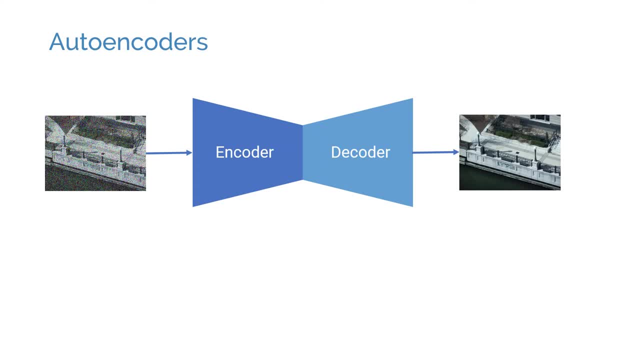 don't have to be identical. For example, the input can be a noisier version of the output. This noise can be introduced artificially. In this setting, the network tries to learn to denoise its inputs. Such a model is called a denoising autoencoder, A typical choice. 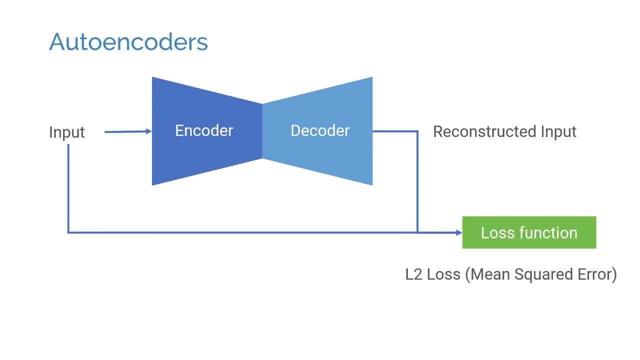 of loss function for autoencoders is the L2 loss. In this case, the learning algorithm would basically try to minimize the loss. In this case, the learning algorithm would basically try to minimize the loss. In this case, the learning algorithm would basically. 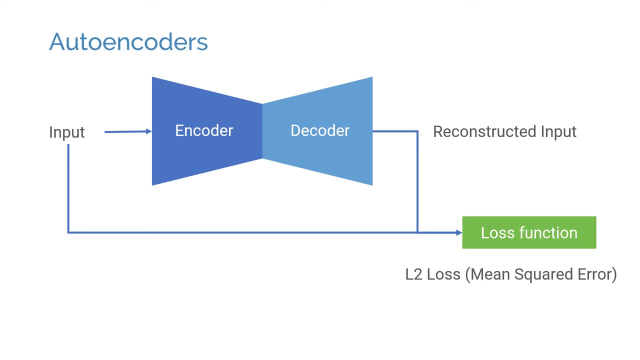 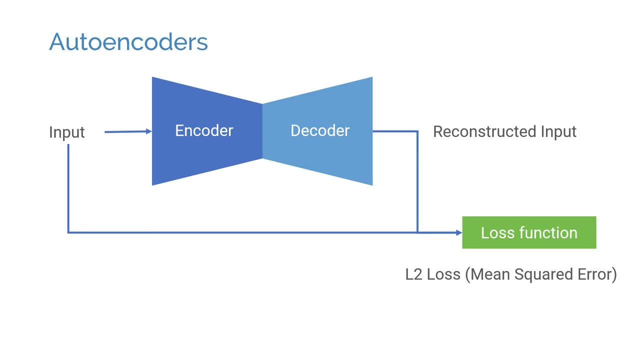 However, my experience is that using the mean squared error on image sets usually results in blurry reconstructed images. Mean absolute error, on the other hand, usually results in crisper images. This might be one of the few domains where L1 loss actually designed. 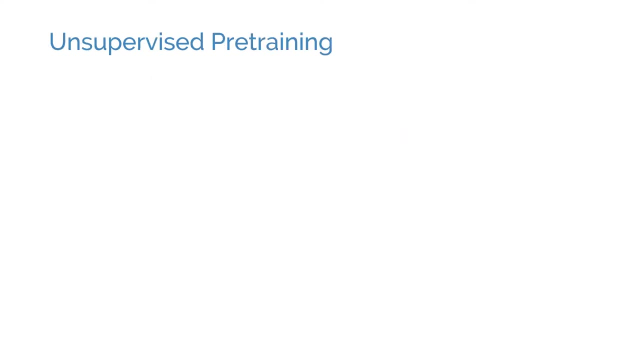 better than L2.. One use of unsupervised learning is to learn representations. For example, if you have large amounts of unlabeled data, but not so much labeled data sized, but the most spicey, It's possible to pre-train a model on the unlabeled data first. 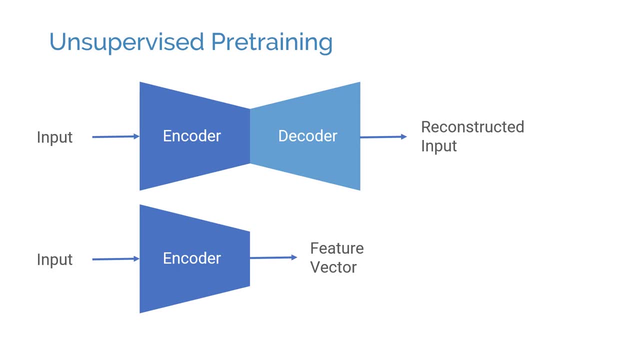 We can use the encoder part of the trained model as a feature extractor, then train a separate model that uses this compact representation as inputs For image data. this approach is not being used often anymore. In case of lack of data, it's more common to transfer features from models trained on. 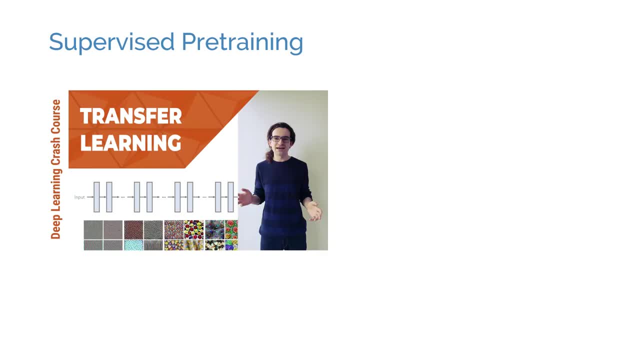 large datasets in a supervised way. You can check out my earlier video on transfer learning to learn more about it. You can find it in the Deep Learning Crash Course playlist in the description below For text data. it's still common to train models on a large corpus of text in an unsupervised 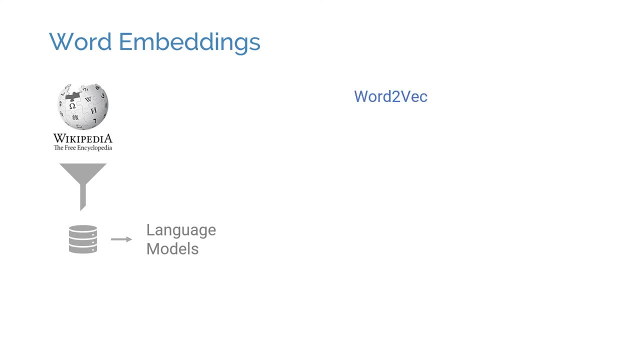 manner. One key example of this is the Word2Vec model, which learns to map words to vectors of real numbers called word embeddings. Before we talk about how word embeddings work, let's take a look at what's a very basic way we can turn words into vectors. 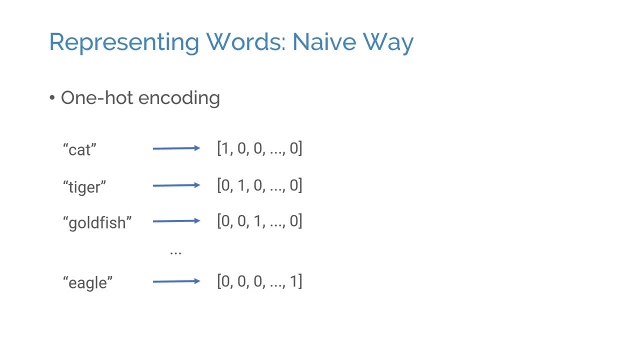 A naive way to represent words as vectors would be to encode them as one hot vector, When each dimension represents one word and all dimensions are mutually exclusive. This representation is not very useful for many natural language processing tasks, for several reasons. First, in one hot representation, all words are equidistant to each other. 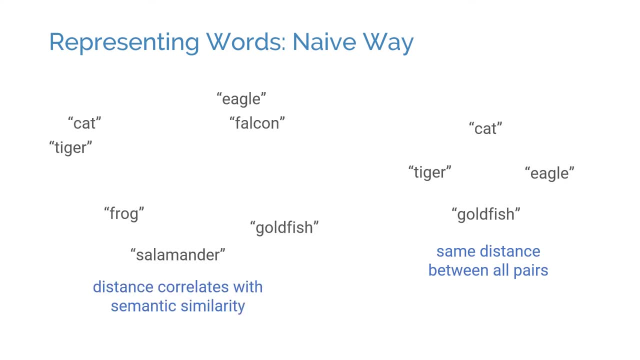 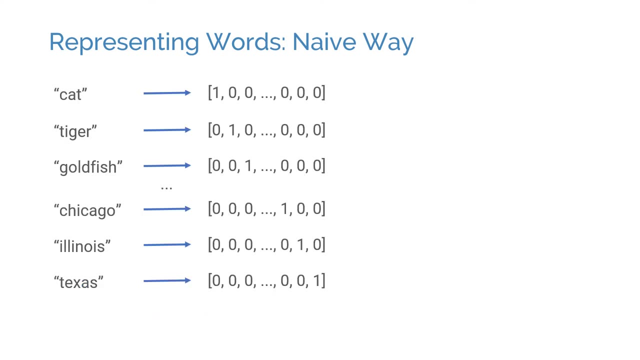 Ideally, we would want the distances between the words to correlate with their semantic similarities. Second, the size of the vectors becomes unmanageable when we have a lot of words in our dictionary. For example, it we have 1 million words in a dictionary, which can CORRELATE with them. 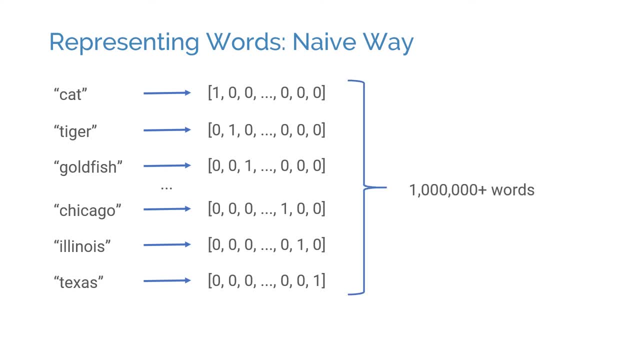 The values that we're using in our dictionary are the exact same values as the words we're using in our working language. So if we see that the size of a word from a word is 1 million, we might want to International represent using vectors of size 1 million. wouldn't be a sensible thing to do. 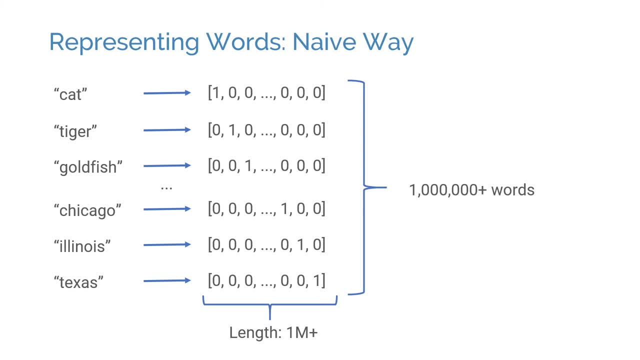 Are there even that many words in English Including the proper nouns? yes, probably even many more than that. So what's a more sensible thing to do then? Assuming that the data can be explained by multiple factors, we can adopt a distributed representation. 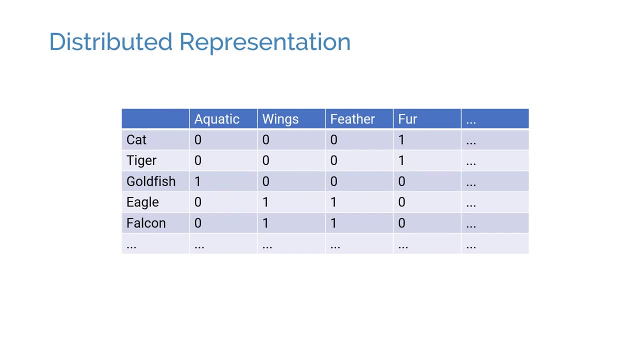 For example, let's say we want to represent the names of thousands of animals such as a cat, tiger, goldfish, eagle, etc. Instead of encoding them using disjoint symbols, we can use a distributed representation, which might have entries that correspond to some of the features that describe an animal. 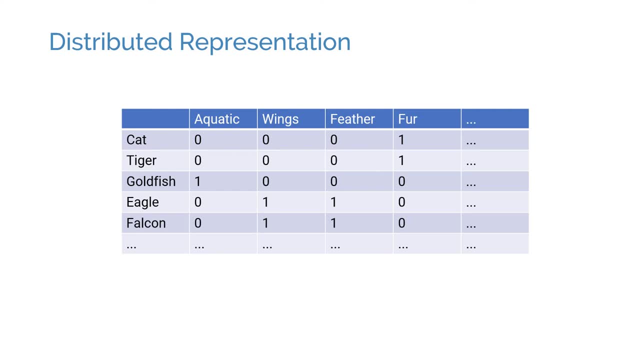 These features might include whether it's an aquatic or terrestrial animal, whether it has wings, feather or fur, and so on. Such a representation would allow for sharing attributes between different words. In this example, the animals that share more attributes will be the animals that share more attributes than the animals that share less. 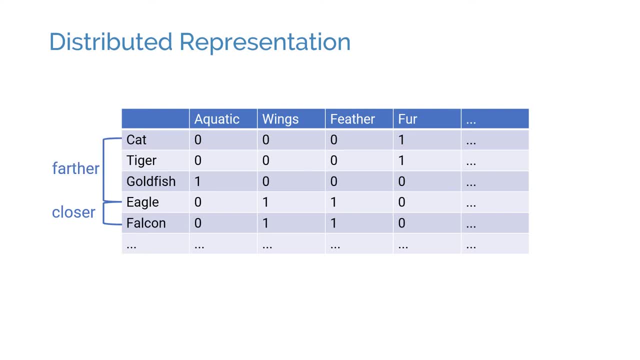 In this example, the animals that share more attributes will be the animals that share more attributes than the animals that share less. The animals that share more attributes will be closer to each other than the ones that share less in the vector space. This representation is more powerful also because it can encode exponentially many words. 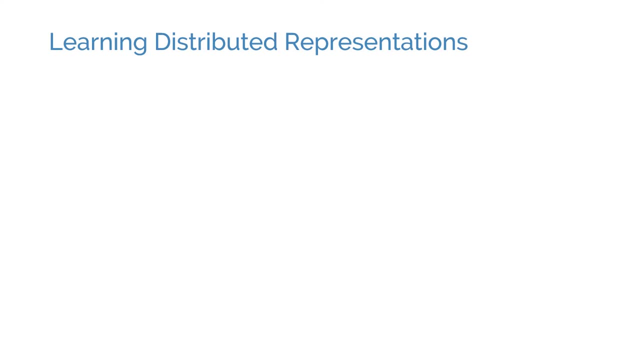 These dense representations can be learned from data in an unsupervised way. Let's take a look at the Word2Vec model, which is pretty much the standard method for learning word embeddings. at the time I'm making this video, Word2Vec attempts to learn the meanings of words and phrases in context. 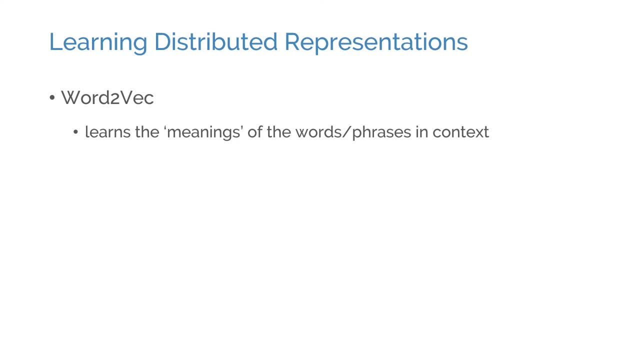 It starts with randomly initialized vectors for each word in a dictionary. Then, given a large corpus of text, it updates the vectors by training the words against their neighbors. For example, if we train a model using a corpus that had sentences that are similar to 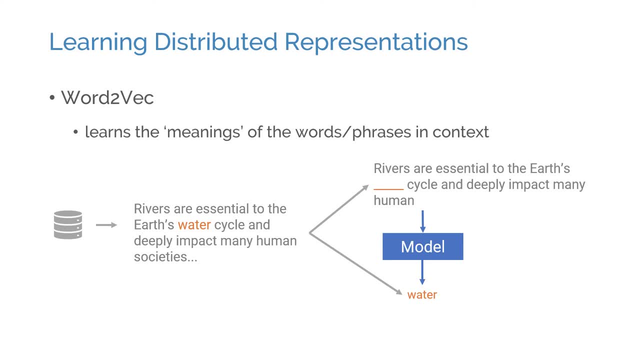 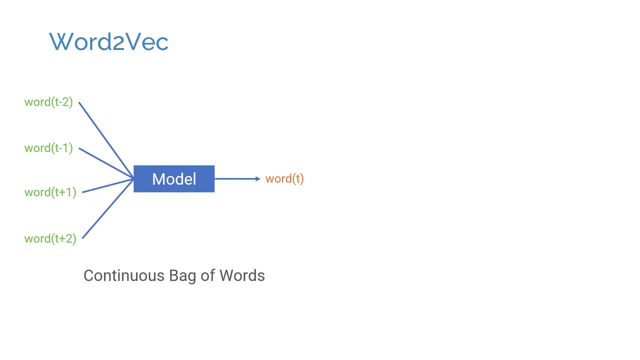 rivers are essential to the earth's water cycle, then the model would be able to learn a semantic similarity between the words rivers and water after seeing them being used close to each other so many times. Word2Vec comes in two flavors. The first type is called the continuous bag of words model, which uses the neighbors of 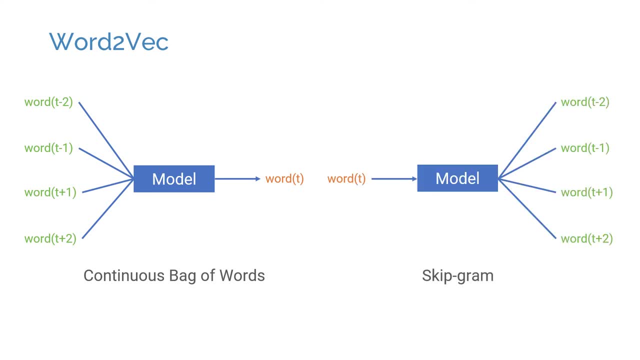 a word to predict the words. The other type, called the skipgram model, does the opposite and tries to predict the neighbors of a given word. Both types seem to capture the semantics of the words well. Let's take a look at some examples. 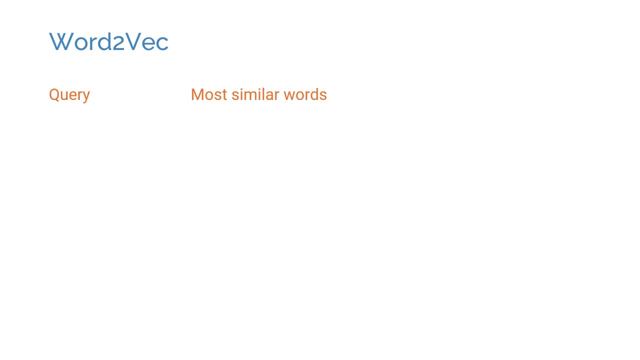 I ran some queries on a model trained on news articles to see what words the model thinks are similar. For example, the word phenomenal was closest to the words incredible, amazing, fantastic and unbelievable. Steve Jobs used to use this word a lot. 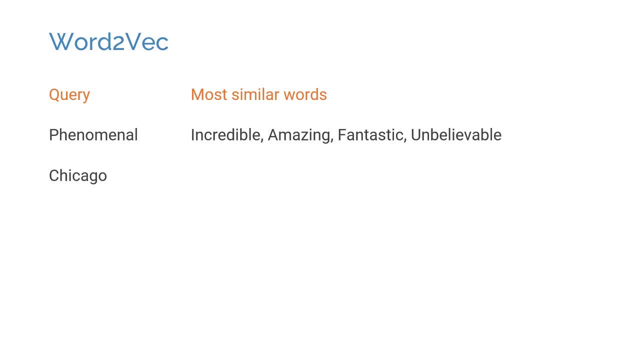 How about Chicago? It seems that it had co-occurred in the news articles frequently with Baltimore, Denver, New York City and Atlanta. Similarly, the word cats had been frequently used with the words felines, cats, pets and kittens. 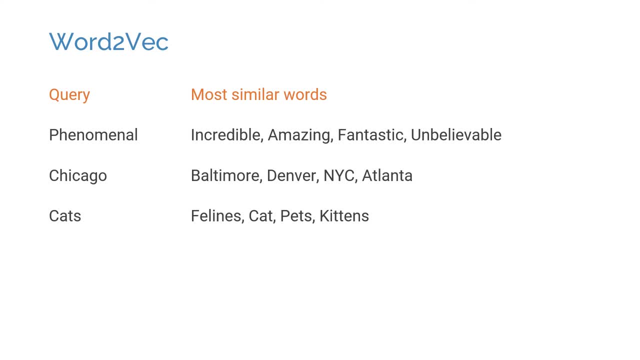 It's interesting that simple arithmetics on these learned word embeddings can be used to capture analogies. For example, using the embeddings from the same model in the previous example, the result of king minus man plus woman gives queen Kitten minus man plus woman gives queen. 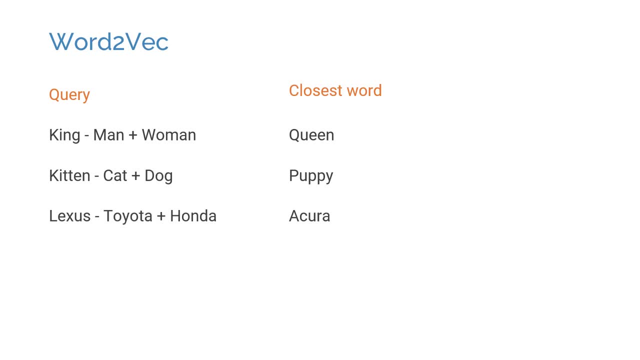 Kitten minus cat plus dog results in puppy. Lexus minus Toyota plus Honda produces a word vector that is closest to Acura. The reason this works is that each direction in the embedding space can learn a different factor that explains the words. For example, one dimension might correspond to whether the subject is male or female. 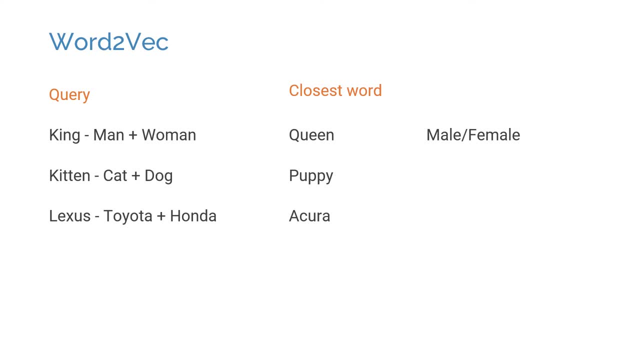 Then when we subtract man from a king, it might change the gender of the word. Another dimension might encode whether the subject is juvenile or adult, Like in the cat and kitten example. There might also be a variable or a combination of variables that correspond to the level. 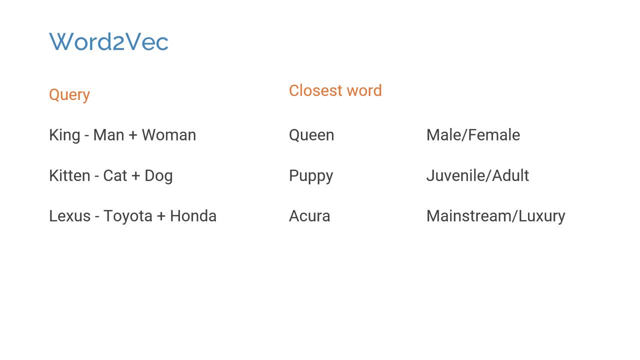 of luxury, like in the case of Toyota and its luxury counterpart Lexus. It's very interesting that these representations can be learned automatically, just by training a neural network on a large corpus of text in an unsupervised fashion. One might argue that this is not unsupervised learning, since the words we train the model. 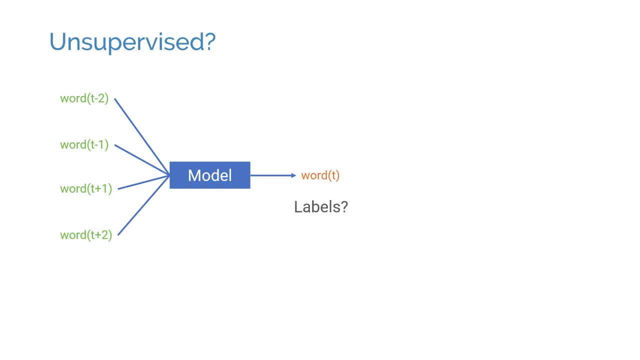 to predict can be considered as labels. Well, The boundaries between supervised and unsupervised learning can get a little blurry sometimes. This kind of tasks can be considered supervised, unsupervised or something in between, depending on your perspective. Another type of unsupervised model that is worth mentioning is generative models. 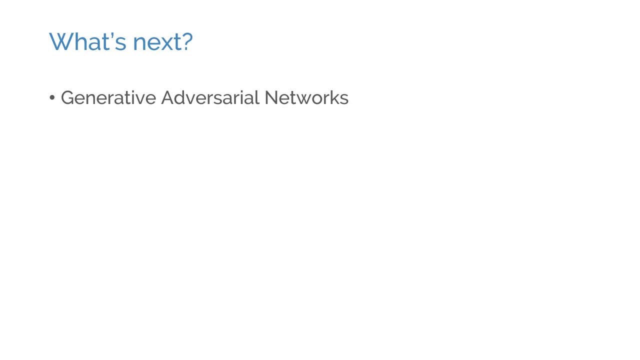 Generative models try to generate samples that are similar to the ones in a training set. Generative adversarial networks, in particular, are one of the recent breakthroughs in this field. I think this is a topic that deserves its own video. I think this is a topic that deserves its own video. 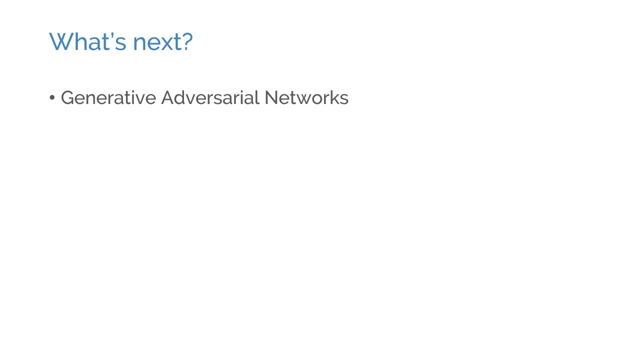 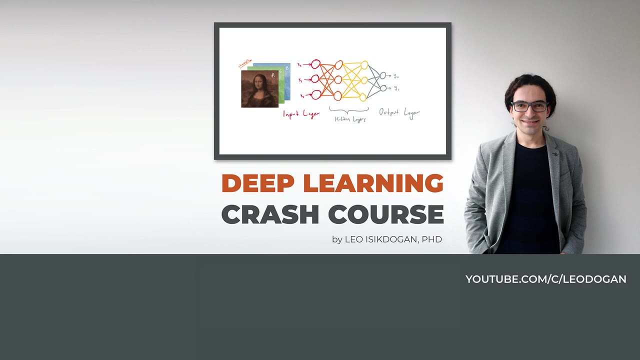 So in the next video we'll talk about how generative adversarial networks work and what makes them so powerful. That's all for today. Thanks for watching. stay tuned and see you next time. 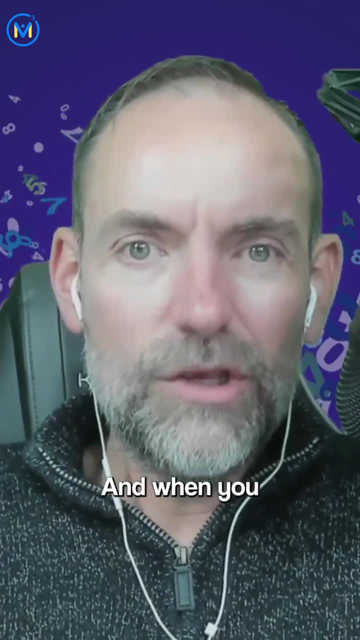 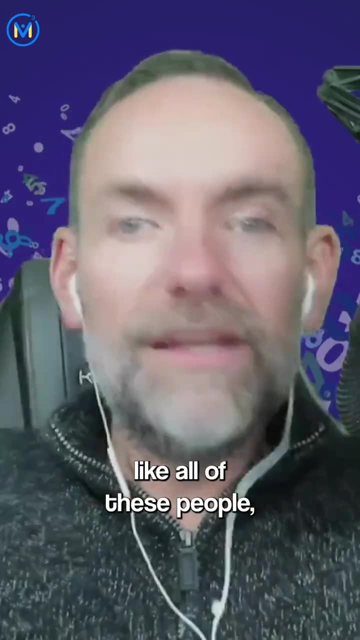 I look at kids like they are our audience And when you have a public speaker or you have someone putting on a concert or you have a standup comedian, like all of these people you are essentially. some people say, oh, teaching or an education, it's not an, it's not an entertainment. 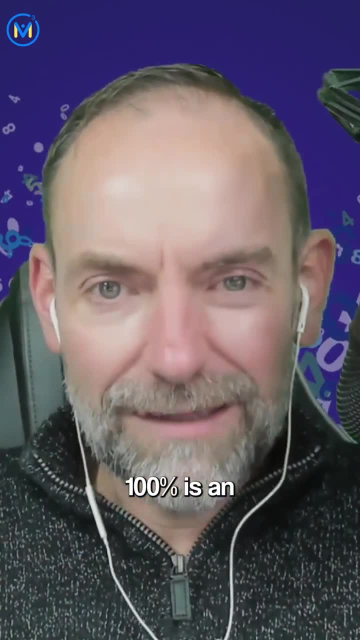 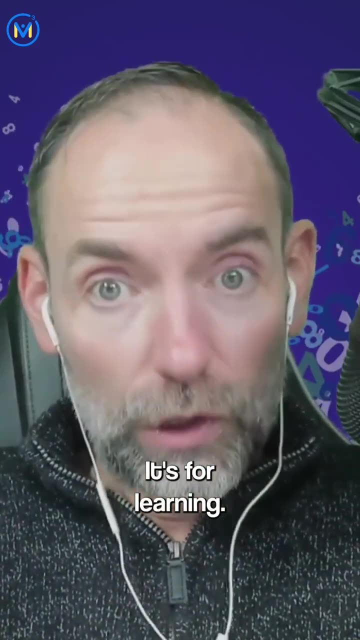 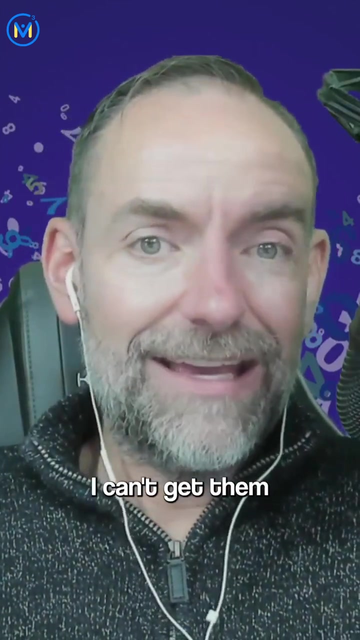 business, but I'm going to say it 100%- is an entertainment business. Now, the end goal isn't just to get a laugh or be interested, It's for learning. But if I can't get students to lean in in what I'm trying to share, that engagement piece, if I can't get them to even just behaviorally, 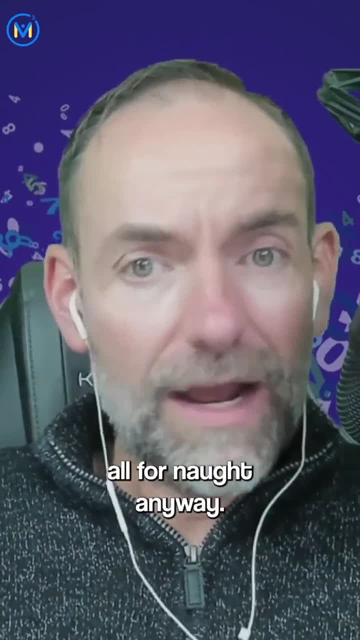 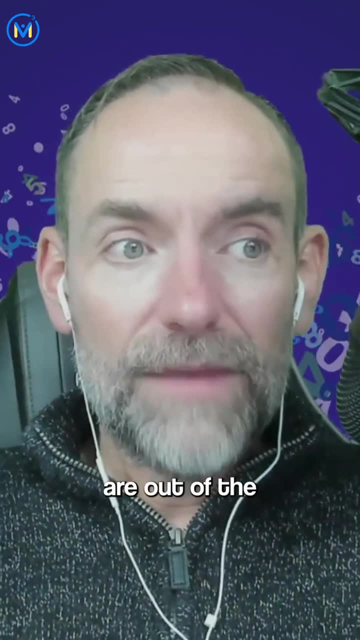 connect with what we're trying to do, then it's all for not. anyway, you know, like we're, we're not going to get to a place where 100% of the students that arrive at school are, out of the box, eager and excited to learn. Now, I think they are naturally eager and excited to learn when.